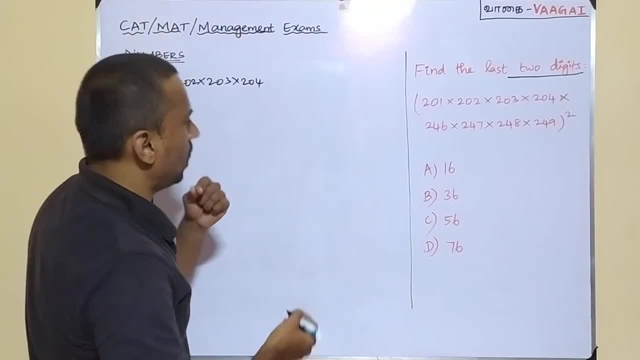 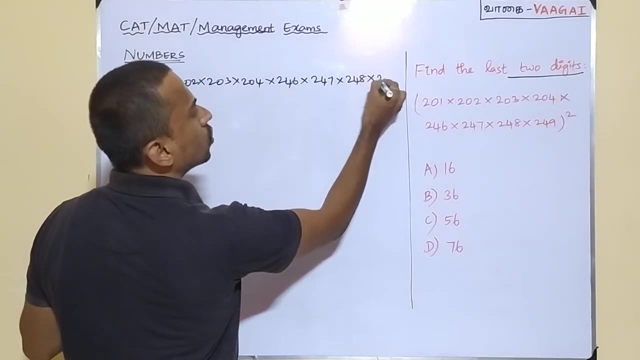 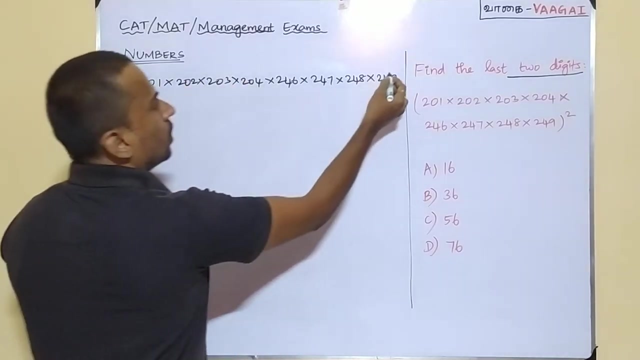 And we have other four numbers. So, continuing the product, we have 246,, 247,, 248,, 249.. So this is going to be the product And here we have got a total of eight numbers and this product to the whole square. So this is what we have, the expression we are given in the question. 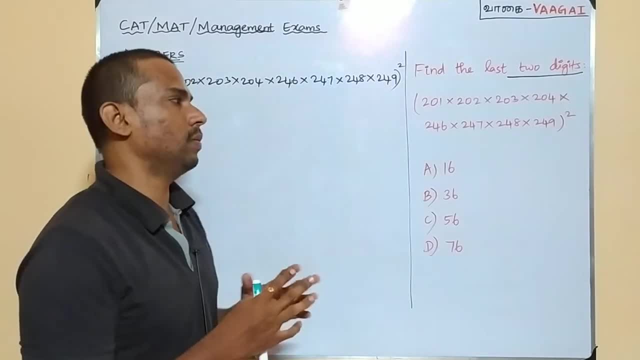 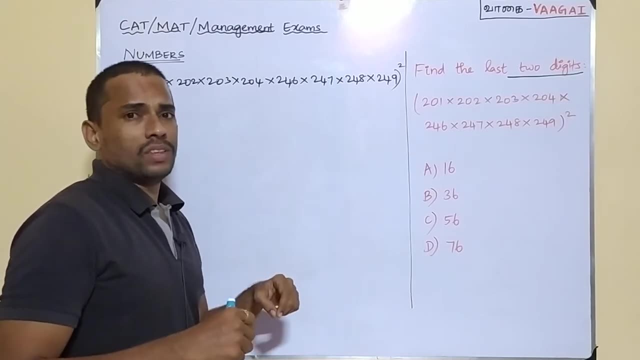 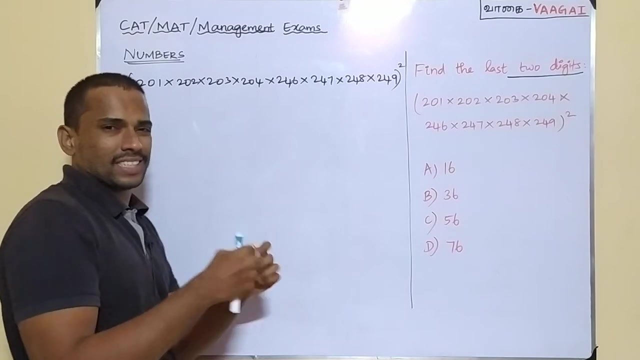 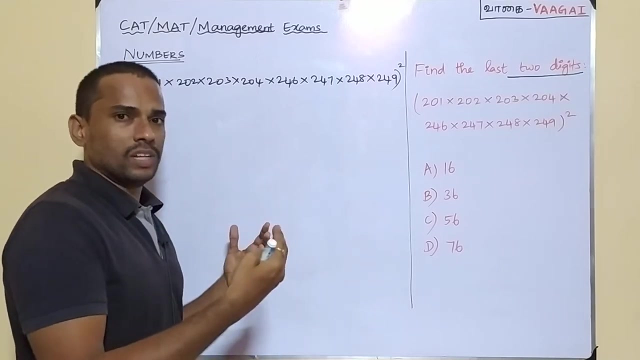 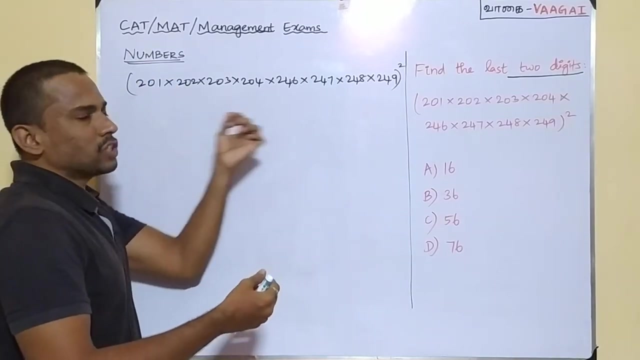 And for which we have to find the last two digits. This is going to be the question. Now, carefully, if you just think of, We are worried only with the last two digits, Only about the last two digits. So in that case, it is better to eliminate the other digit except the last two digits. So, wherever we have these numbers, out of all these numbers we will just eliminate, We will just remove the other digit, Okay, Which we are not concerned about. Okay, So in that case we will take only the last two places alone. That is sufficient for us to get the answer. So in that case, we can reduce the same expression to: 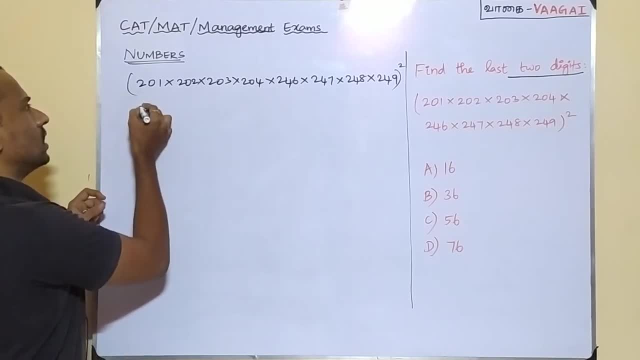 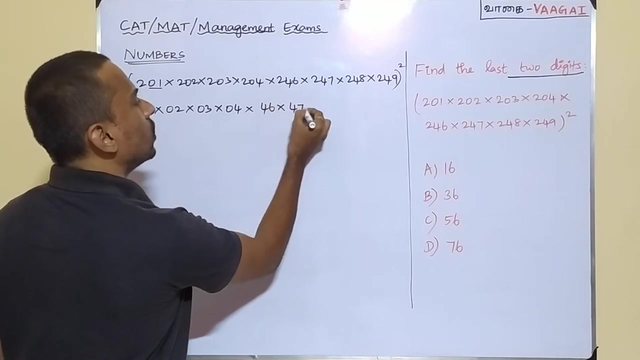 So in that case we can reduce the same expression. to Just listen How I can rewrite it is: Just take out of this 201.. Just take the 01 alone, Because we need the last two places only, Right? So in that case we can reduce this entire expression. in a similar way, What we can do here is I can rewrite it as 01 into 02, into 03, into 04, multiplied with 46, into 47, into 48, into 49. The whole square. I hope you are able to understand what I am doing here. 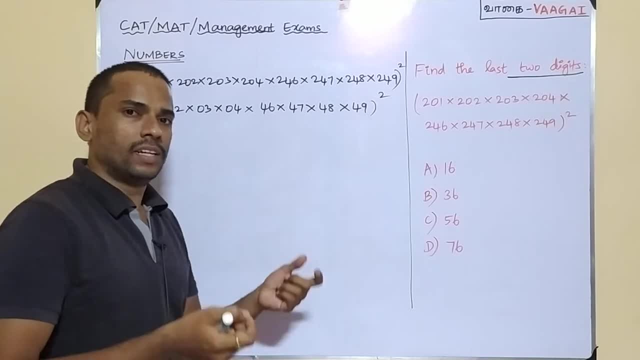 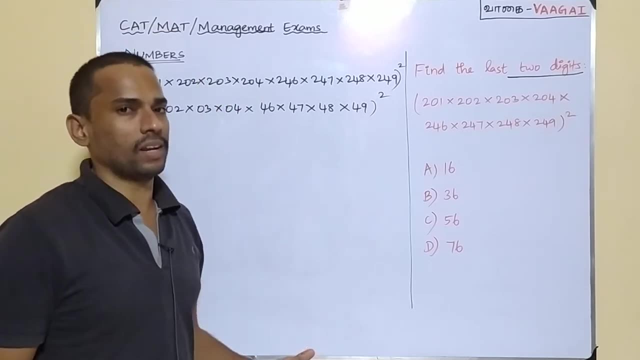 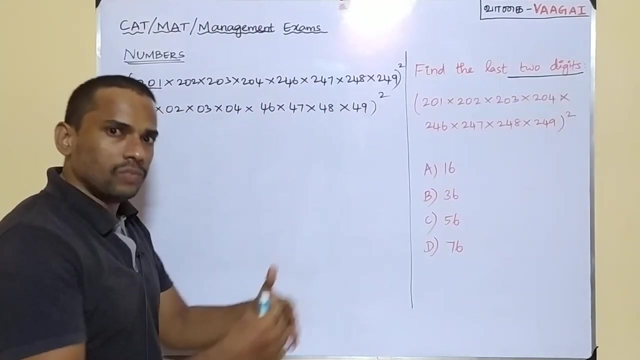 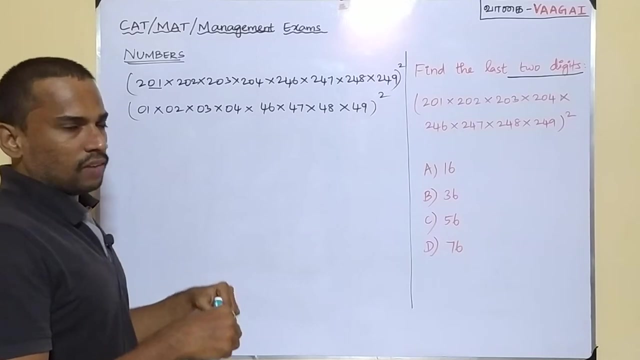 Since we are asked to find only the last two places, it is enough to play with the last two digits, That's it. Okay, Our answer won't get affected. We will be still getting the same correct answer. That is the reason. So we will now try to find the last two digits of this expression Equivalently. that will be the answer for the given question also. Okay, Alright, Yes, Now again coming back, we are again having the same eight numbers, but only with the last two places. Let's do something here, Okay. 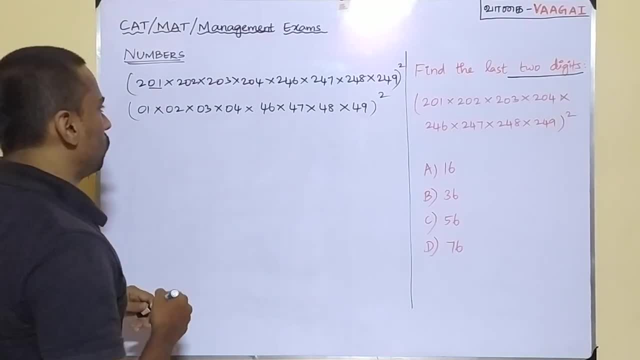 Let's do something, Let's segregate, Let's group the terms, Okay. So, if you see, here we have got the first four numbers, First four terms. Okay. So here we have 01, 02, 03, 04.. Now I think this case it would be very easy for us to get the last two places Right, Since our numbers are too easy. we can directly multiply these numbers Because we have only small numbers here, Right. So it is like 1 into 2, into 3, into 4.. So what about this product? it will give you 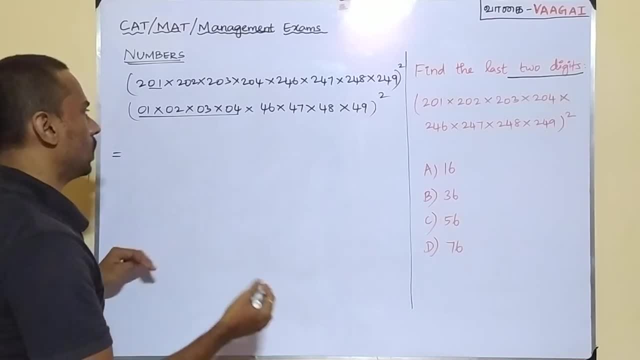 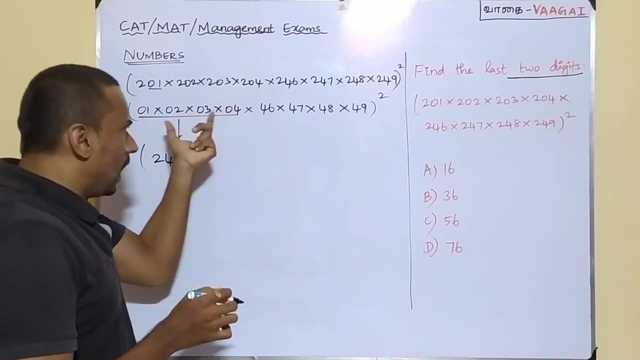 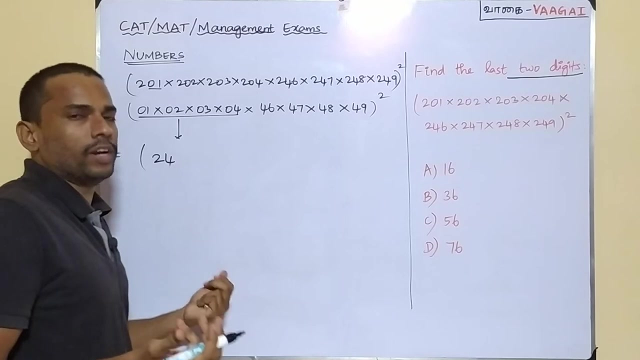 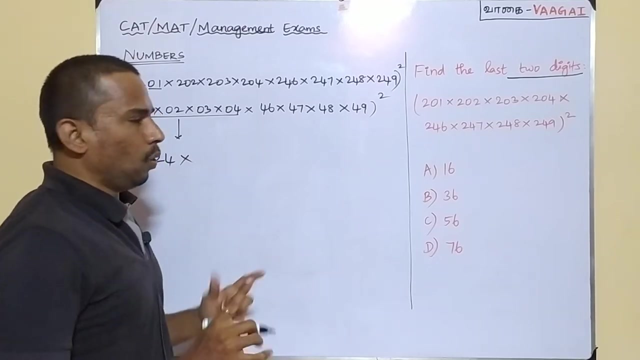 12, twos are 24 and 24 ones are is 24.. So that means this will simply give you 24.. Okay, So the first four numbers when grouped, that is giving you the product 24 and of course that becomes the last two digit itself. Okay, For this group the last two digit is going to be 24 only, So no issues with that. So 24 here multiplied by, multiplied by. Now comes the challenge. Okay, Now we have the other four numbers here: 46,, 47,. 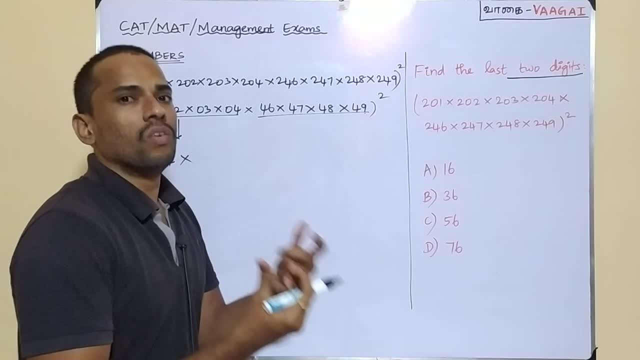 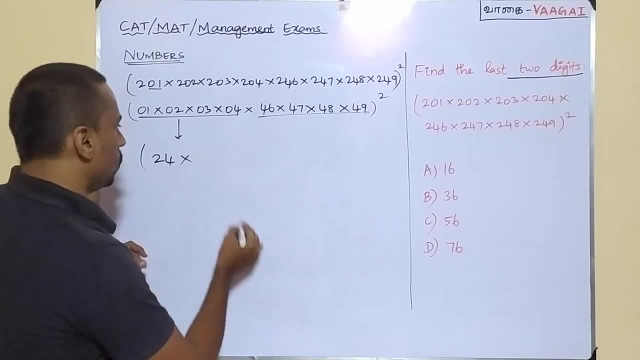 48, 49. So those numbers are to be multiplied, for which we need to find the last two places. That is going to be a quite big challenge, So let's do that carefully. Okay, Now, what I will do here is: let me just make a small space here so that the answer, what I get for 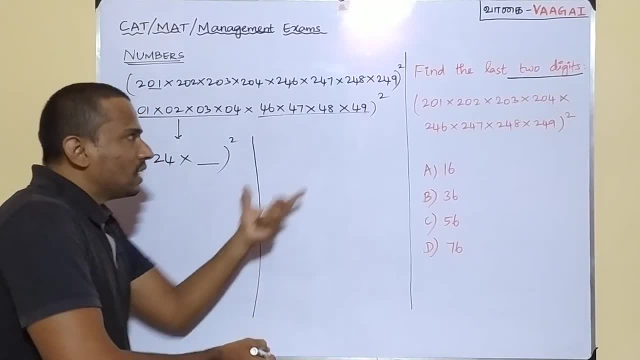 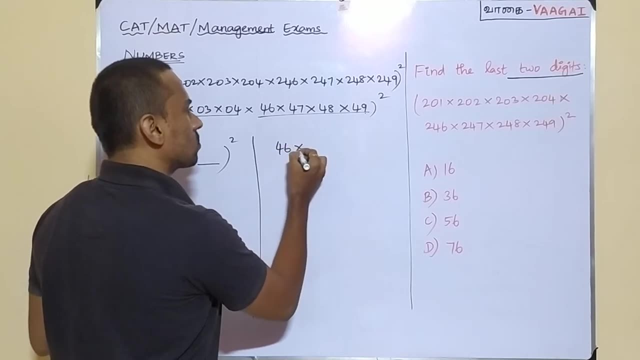 this one. I will note it here. Okay, Fine. Yes, Let's try to work this calculation separately. Okay, Alright. Yes, So if we rewrite those numbers 46, 47,, 48 and 49.. Okay, Fine, Yes. 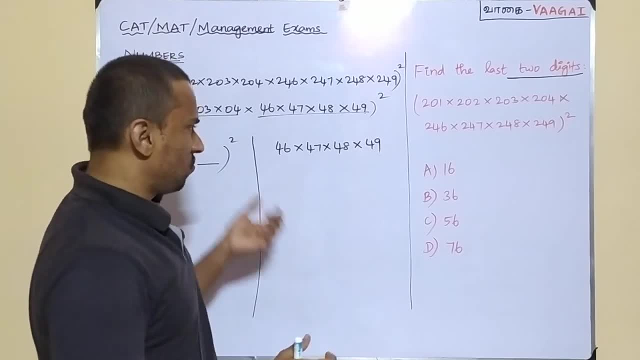 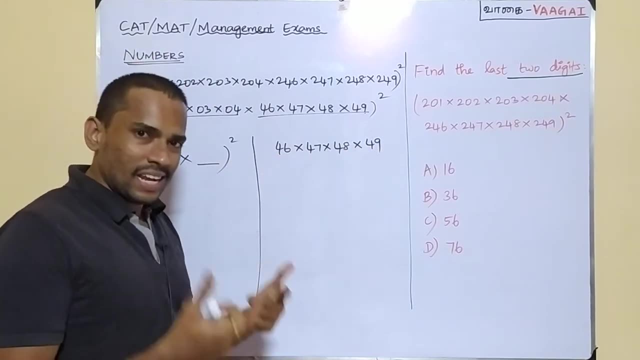 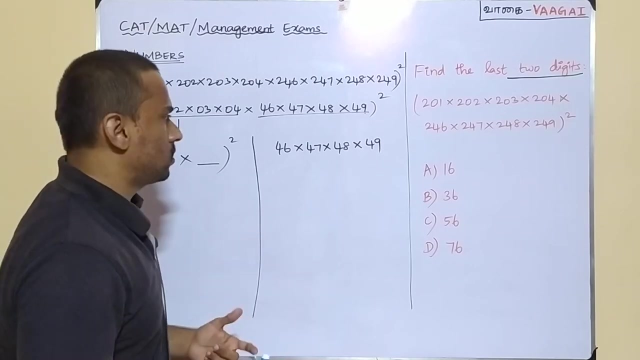 So now we need to find the last two places for this product. That is going to be the challenge, Alright? Yes, Now, if you see these numbers, we can rewrite them. as We can rewrite them, as, See these numbers, they are much closer to the round number 50.. Right, Yes, They are. 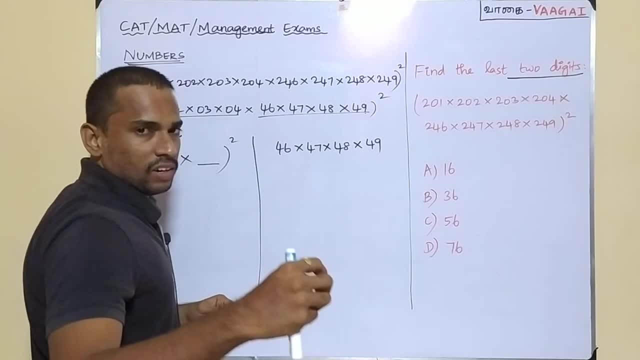 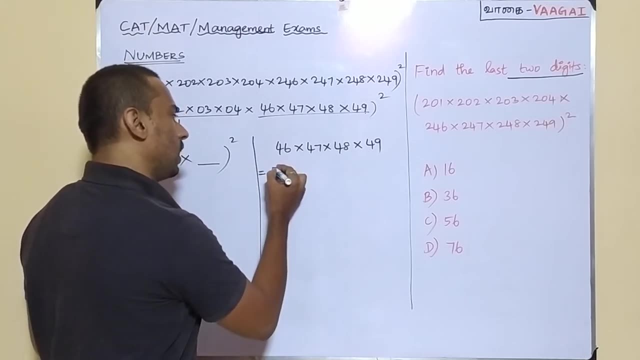 much closer to 50.. Right, So in that case, what I will try to do here is let me rewrite these numbers something like this: Okay, Just look at it carefully. So this 46, I am going to write it as 50 minus 4.. Next, this one, 46.. This 46 is written like this: for 50 minus. 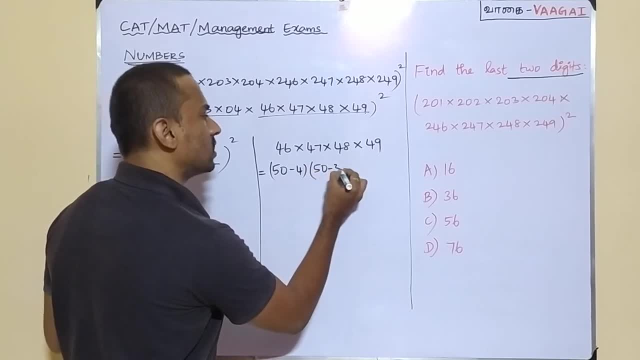 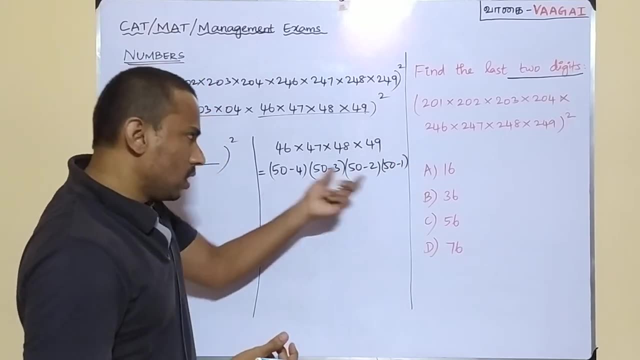 4. This 47, I am rewriting it as 50 minus 3.. Next, this is 50 minus 2 and this is 50 minus 1.. Okay, Fine, Yes, Maybe it looks in a cool way. that is the reason I am rewriting like: 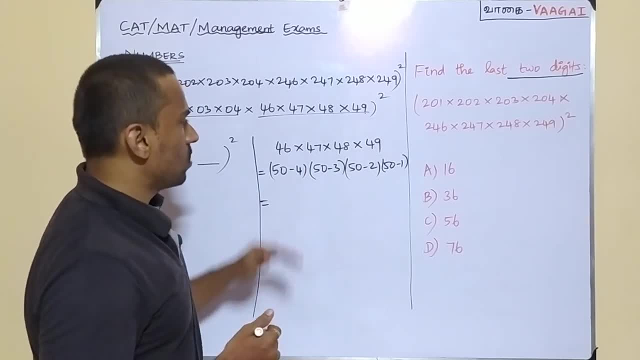 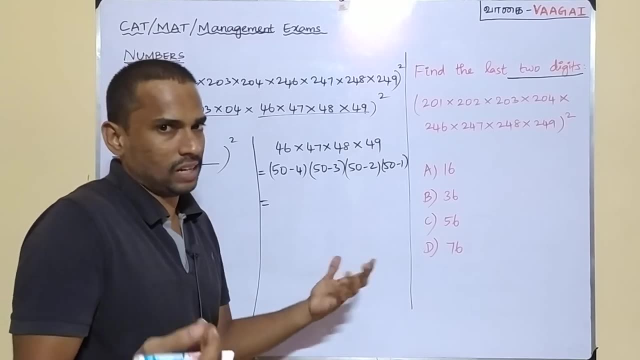 this. Okay, Now, continue this. So now, if you see, we have rewritten these numbers like this, Now, if you play with this expression, it would be more easy for us to find the last two places. That is the reason. Okay, Alright, Yes, Now we have got four terms here. Again, let me. 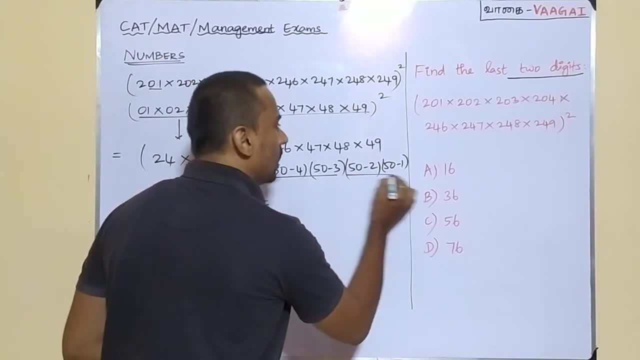 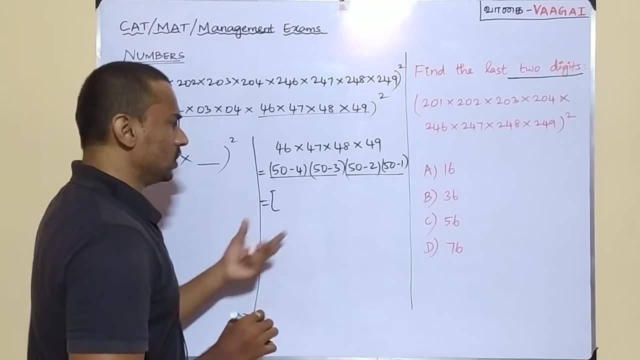 group the terms. I will take the first two terms and next the last two terms. I will take it like this: Now, when you try to multiply the first two terms, what happens? Can you just see here? This will simply become: This is like two numbers, I mean like there are. 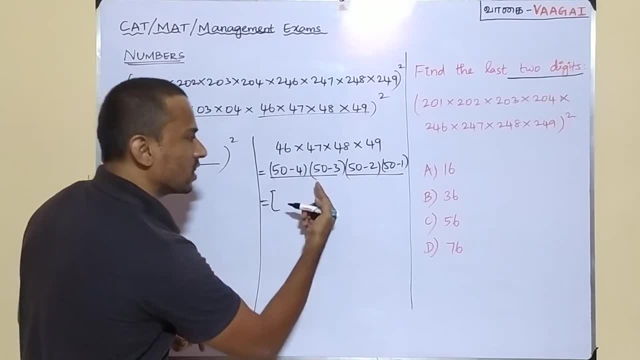 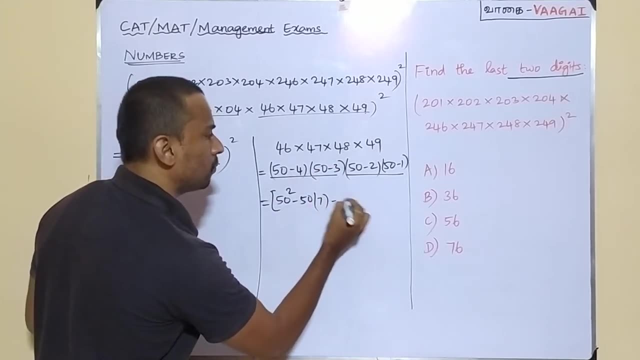 like two factors of a quadratic expression, Is it or not? So 50 minus 4 into 50 minus 3.. This will simply give you 50 square minus 50 into what about 4 plus 3, which would be 7 minus. I am sorry it will be plus, because minus 4 into minus 3 will be 12.. I hope you. 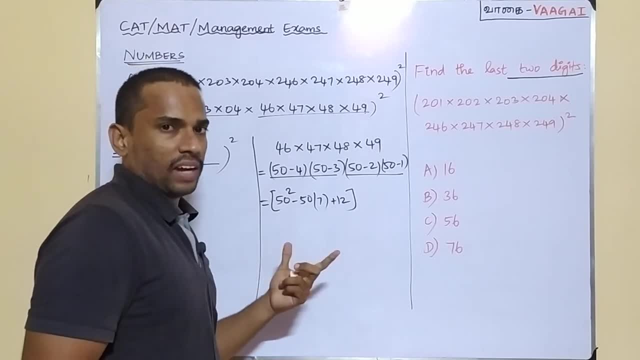 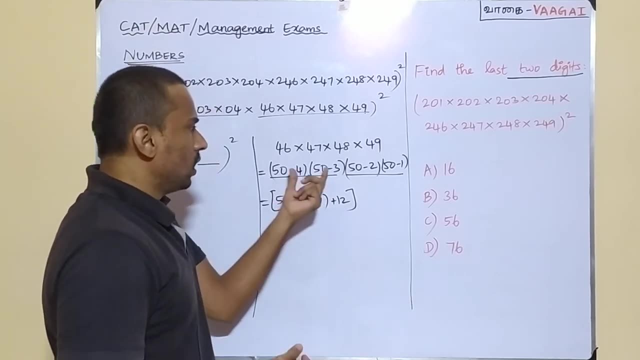 understand this. Okay, There are two like two factors. they get multiplied, which is what I have expressed here. So it is like x square 50 square minus x into the sum of the. it is like those two numbers are like the roots. Okay, 4 plus 3, which is what is this? 7 and 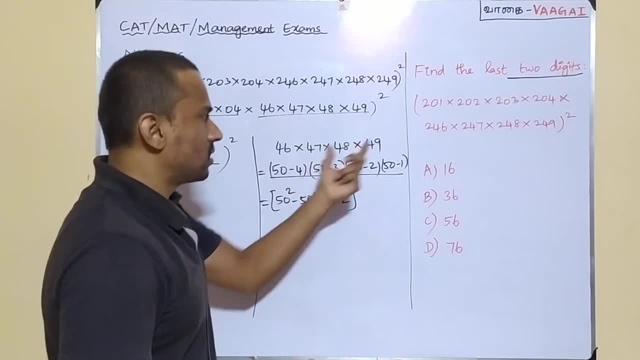 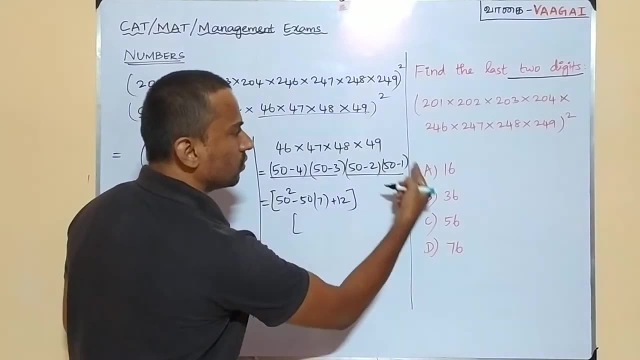 minus 4 into minus 3, which is giving you this plus 12.. Okay, Repeat the same process for the next two terms, also Here. what we get is here Again, if you carry the same process, you here 50 minus 2 into 50 minus 1.. Here you will. 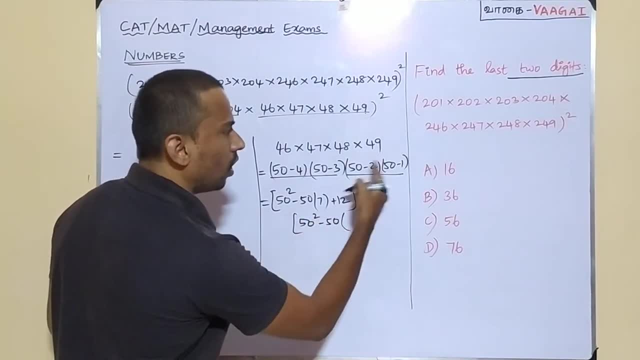 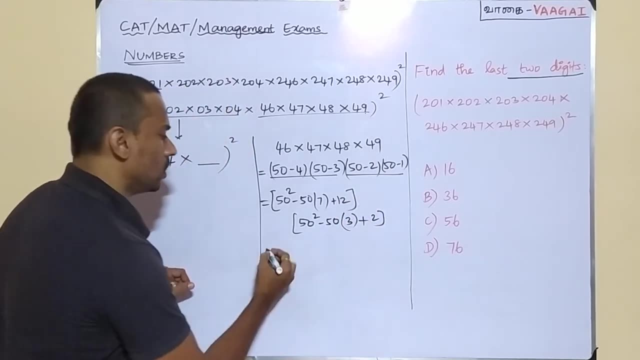 be getting 50 square minus 50 times of this will be 2 plus 1, which will be 3 plus plus 2. ones are 2.. So this is what you will be getting here. So continue this process. Continue this process Again. what I can do here is again, we will just worry about only the last. 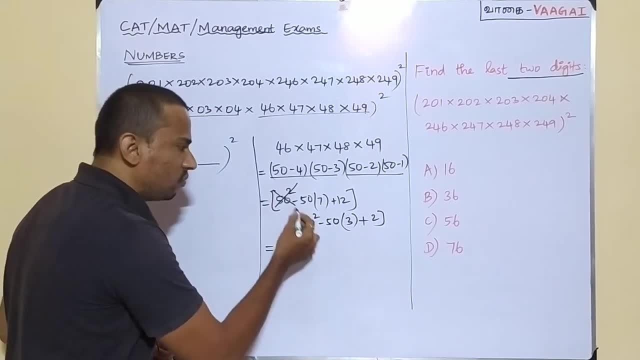 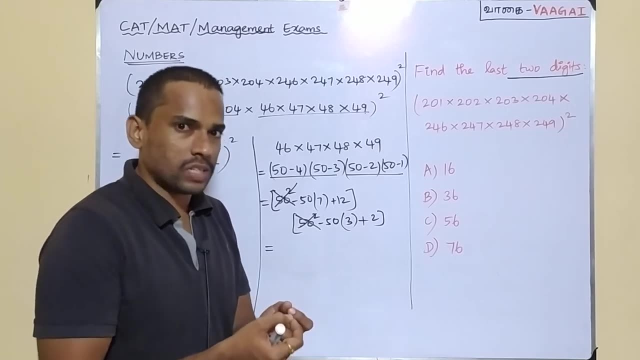 two places. Right, Okay, So in that case we can eliminate this 50 square and 50 square. Anyways, 50 square is going to be 2500.. 2500- last two places. it is going to be again double 0.. Is it or not? So that will not make. 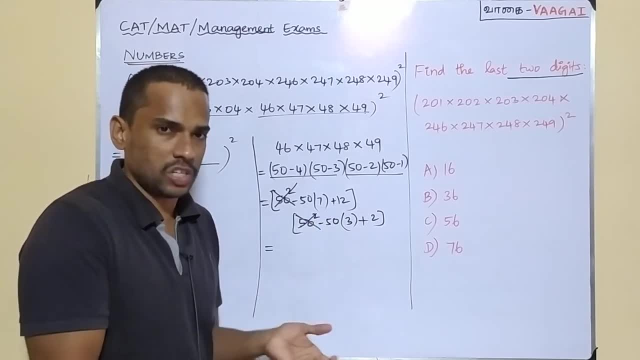 our problem to be. I mean, like it won't give you any change there. For that reason, we will just eliminate that. We will worry about only the expressions where the last two digits involve: make the change, make an impact. That's it, Okay. So now, when you come here, we have 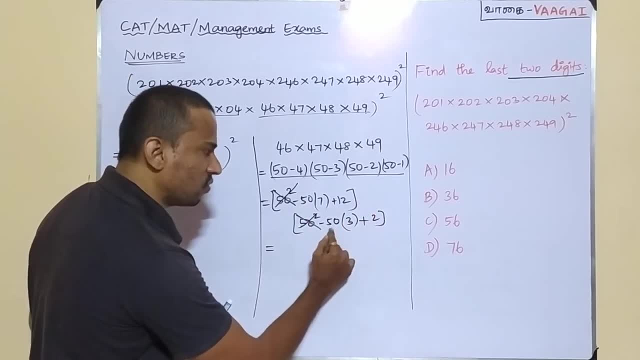 50 into 7 plus 12 minus 50 into 7 plus 12 minus 50 into 3 plus 2.. This is all we have here, So in this case we will carefully work it out Again. I can make a quadrangle, Okay. 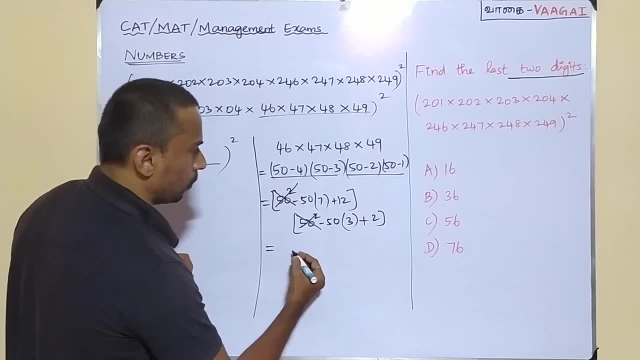 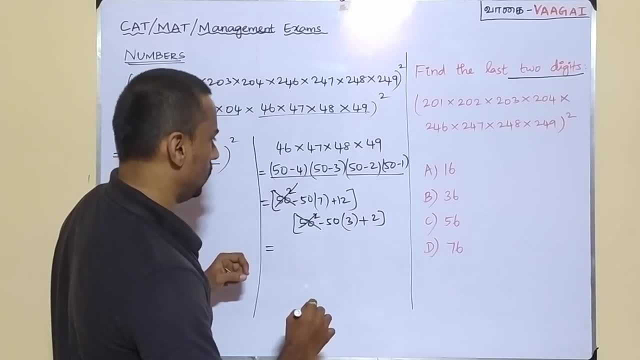 like this. Let me try to do it like here. we have like. we can even play it like this, because minus 50 into 7 will be like a minus 350.. Right, So it is again minus 50 plus 12, and again continue here. Minus 50 into 3 will be like minus 150. it is like again minus 50. 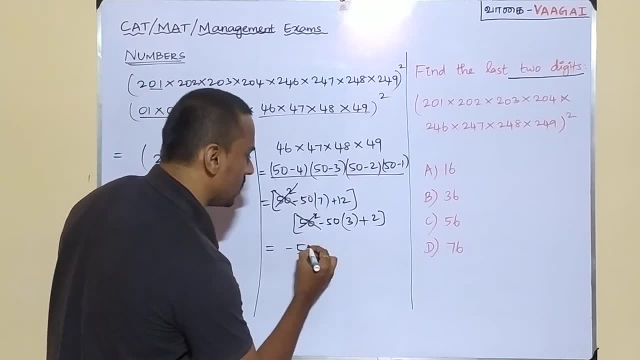 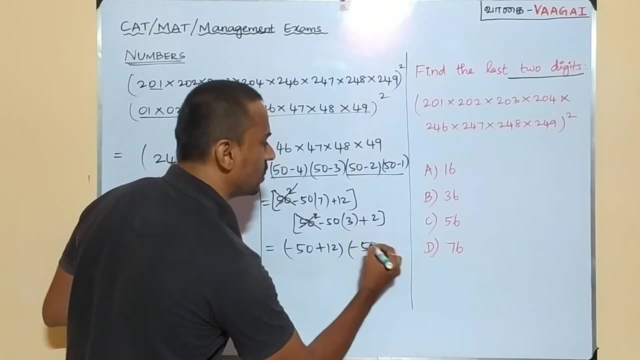 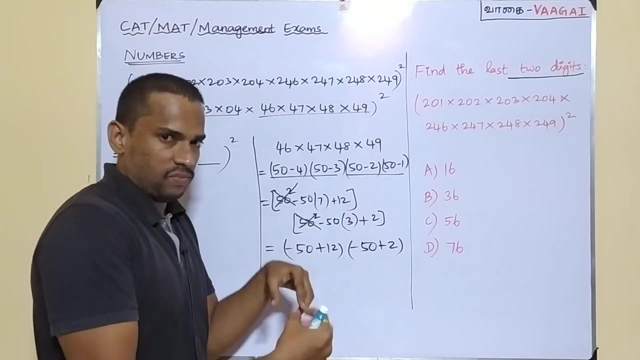 plus 2.. Okay, Let me make it clear so that it won't confuse you. Okay, So my first answer is super simple, right? So let's try again. Alright��, you much. Let me just repeat the process, what I have tried to do here. Here it is minus. 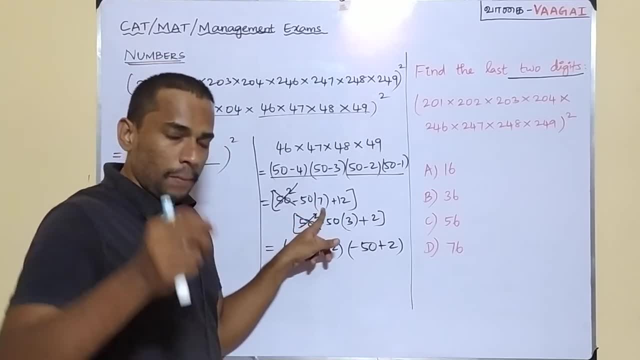 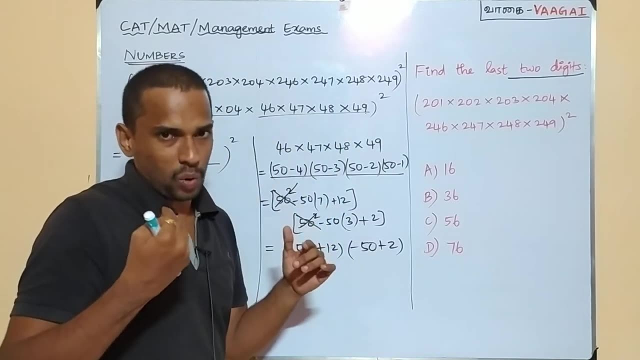 50 into 7.. Is it or not? So minus 50 into 7 will be minus 350.. Again, from that minus 350, I am removing that 3, that 300.. Why? Because I am very much caring. I am just caring. 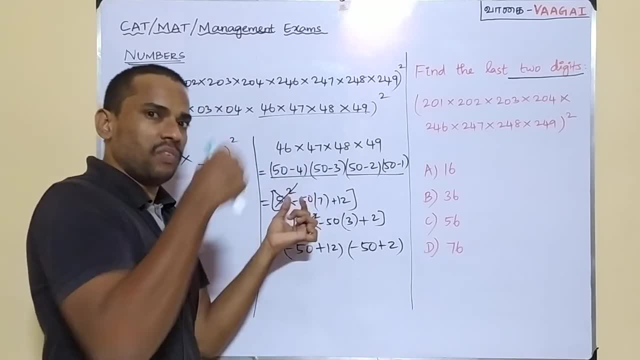 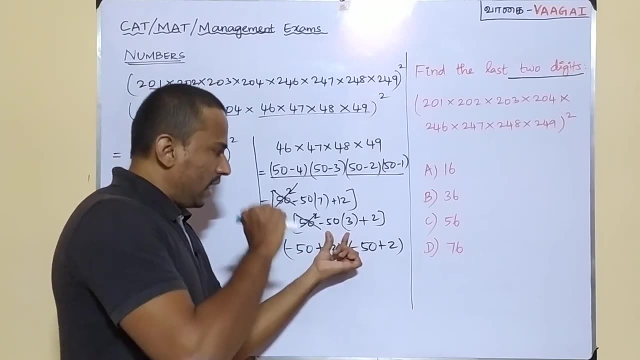 about only the last two places For that reason is what? From that minus 350, I am removing that 300, taking only this minus 50.. Same thing I am doing here: From this minus 50 into 3, which is going to be minus 150,. I am worried only about the last two places, which. 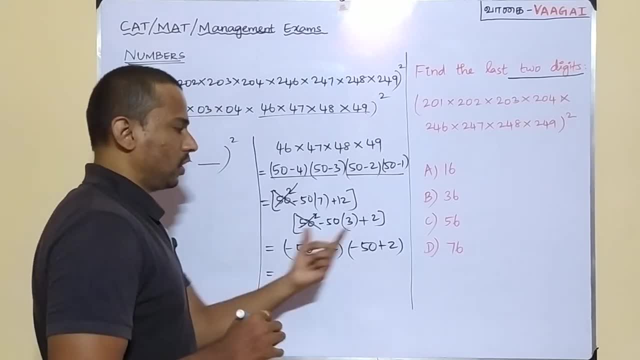 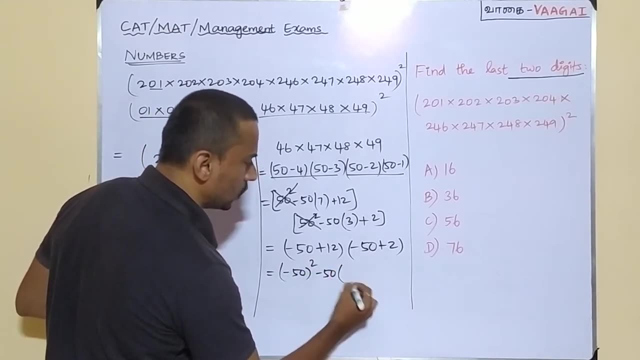 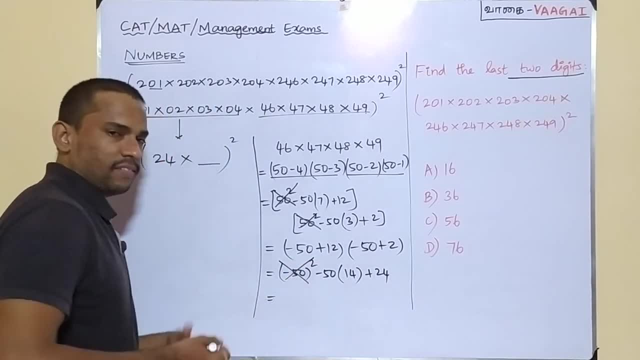 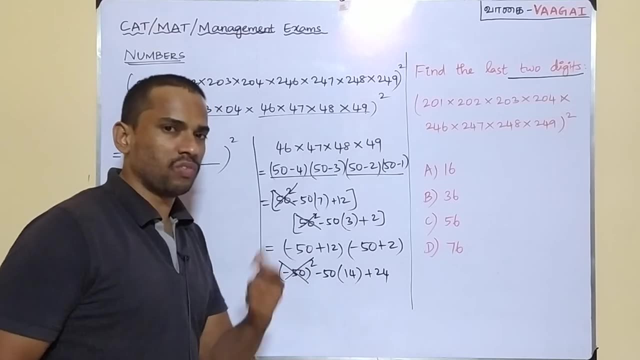 this is minus 50. So this is minus 50. Okay, So again I can eliminate this one. Anyways, this is going to give you double 0. So you can eliminate it, and here you have minus 50 times of 14.. What is minus 50 times of 14?? It is going to be minus 700, right? So? 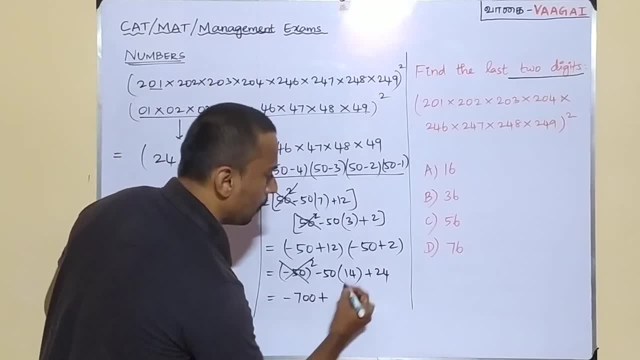 this is going to be 700- and again, it is not going to worry you much- plus 24.. So, finally, what you get here is, again, you will get the last two places to be simply 24.. Why? Because you see, here this is exactly 700.. 700,, in this sense, last two places, is going to be: 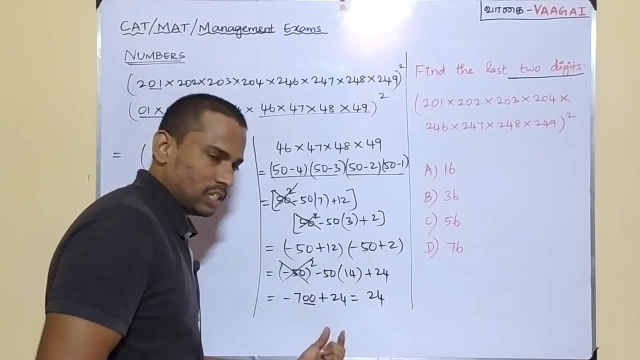 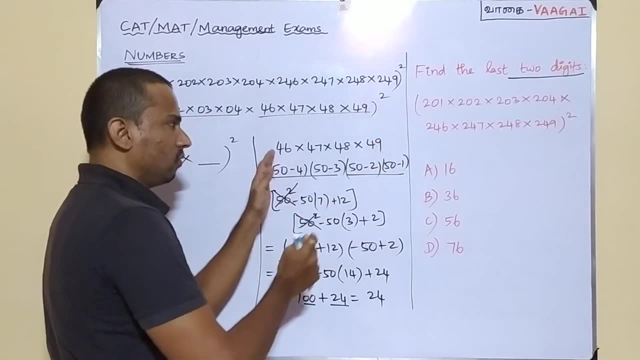 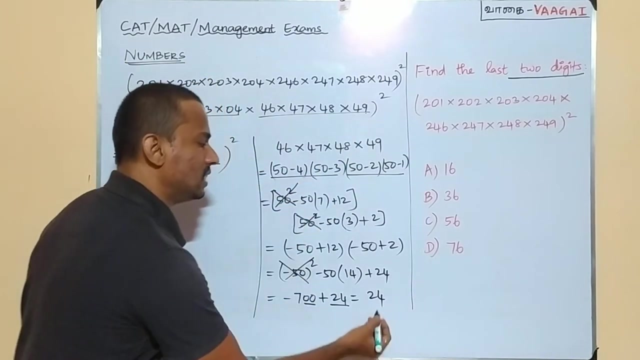 be double zero only so in the case it is not going to affect your calculation. so you are simply left with 24 here. so that means this product, i mean the product of these four numbers: 46, 47, 48, 48 is going to end up with the two digits, again 24. so just take this 24, put it over here, so here. 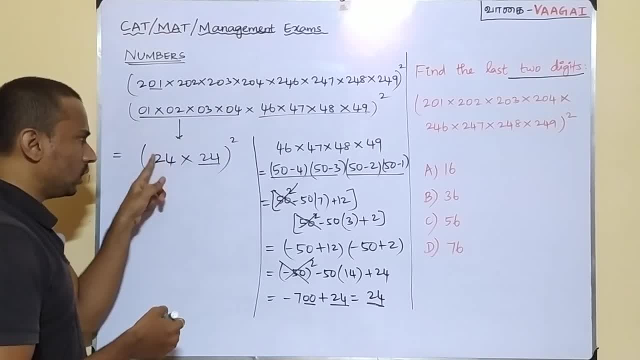 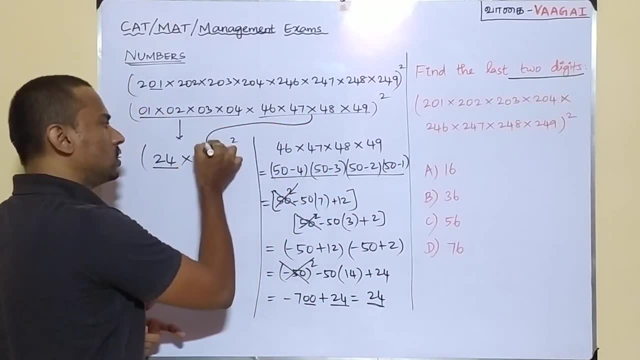 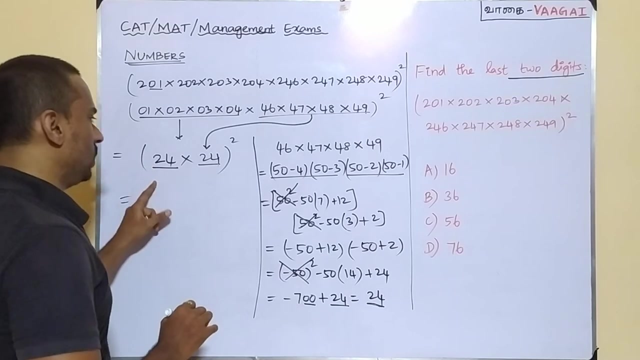 we have the first four numbers product is giving you the last two places to be 24. you have taken it and again, after all these calculations, the last two places of this product. this is again giving you the same 24. we have noted it. so our question now simply becomes 24 into 24, the whole. 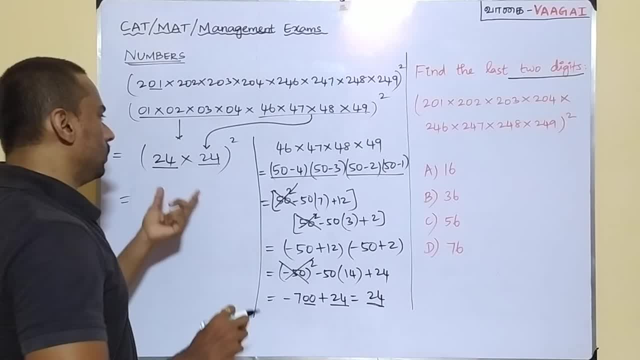 square. okay, now we are worried only about the last two places of this simple calculation. this won't be much complicated for us, so hereafter we can carry out and easily finish off the problem. so, 24 into 24, the whole square. this is what we have right. so basically, what is 24 into 24? 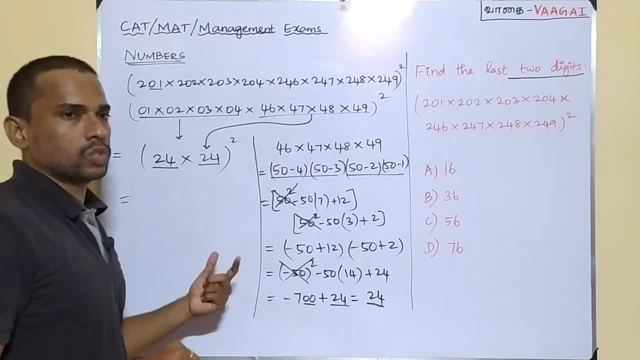 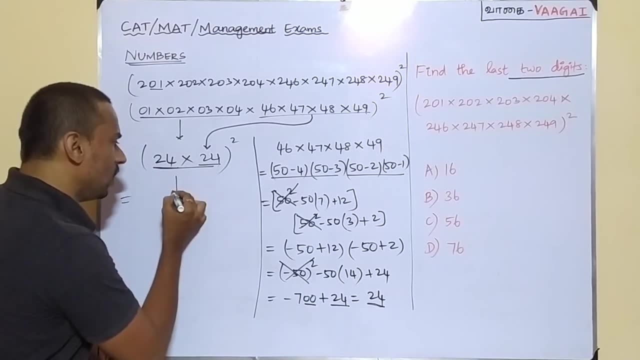 24 square, it is going to be what? 24 square is going to be 576, right? so 24 into 24 is going to be 576 and of course, this will give you- okay, maybe, if you want, i will separately note it down- 24. 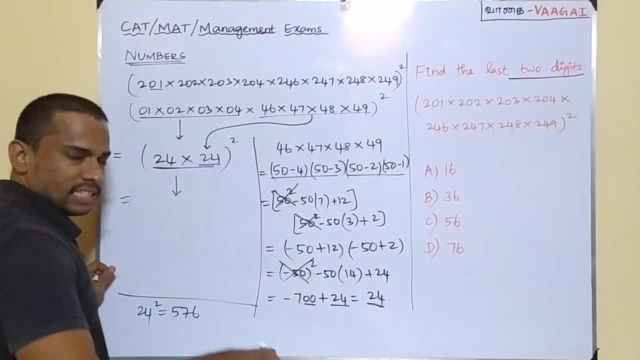 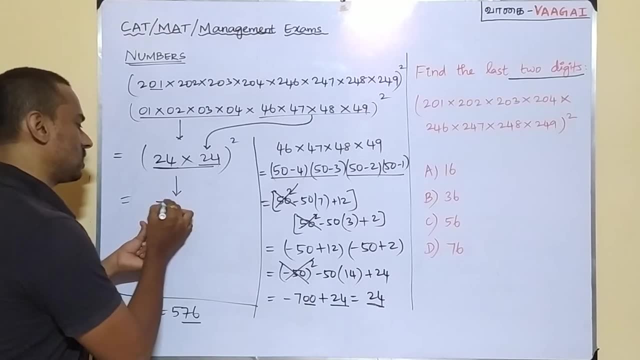 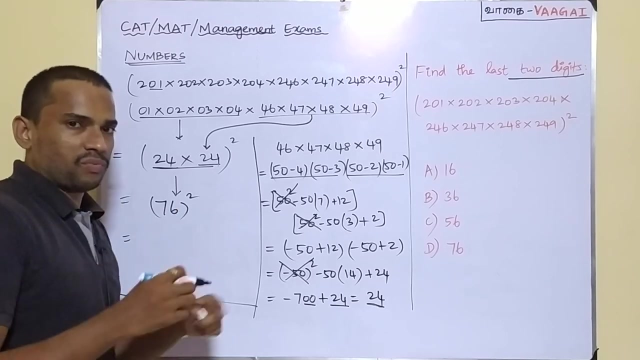 square is going to be 576 and again, since we are worried about only the last two places, it is enough to consider only this last two places, which is 76. so 76 square, that will what comes, that will only come here. so 76 square. and final stage, last one more step we need to do just again: calculate what is 76. 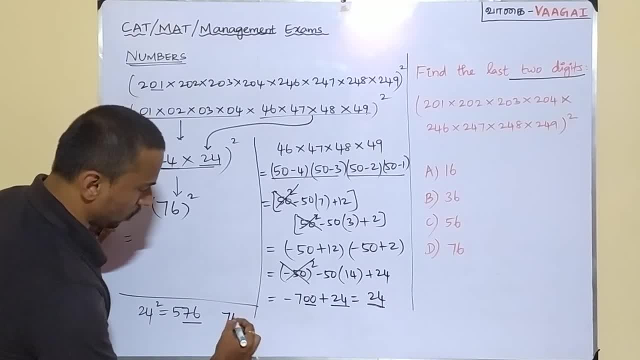 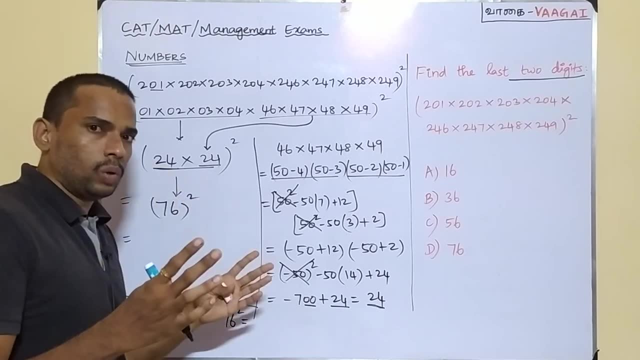 square. 76 square is going to be what? so 76 square? if you want to calculate, what i can do here is: or again, you can even rewrite this 76 square as something else, or if at all you don't want to complicate the process, you can simply calculate what is 76 square. so 76 square is going to be. 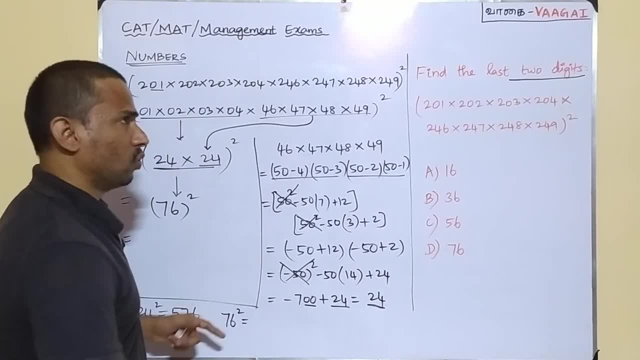 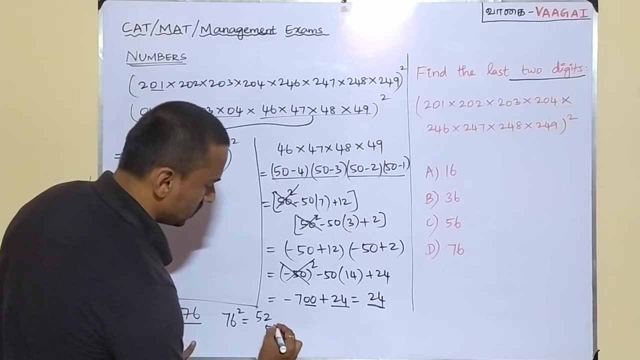 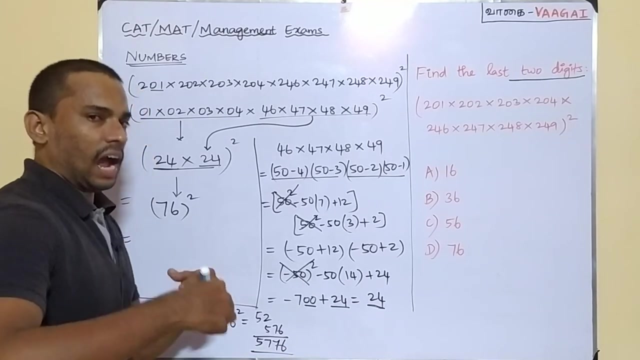 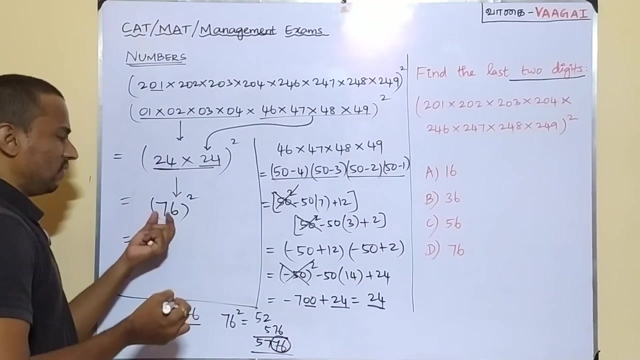 like 76 minus 24, which will be 52, and then it is going to be 576, 576. so the answer is going to be 5776. so 5776 is going to be the answer and, of course, again, we are worried about only the last two places, which is going to be 76. so this 76 square. 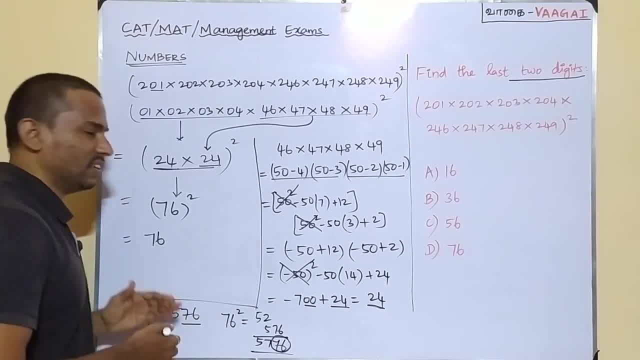 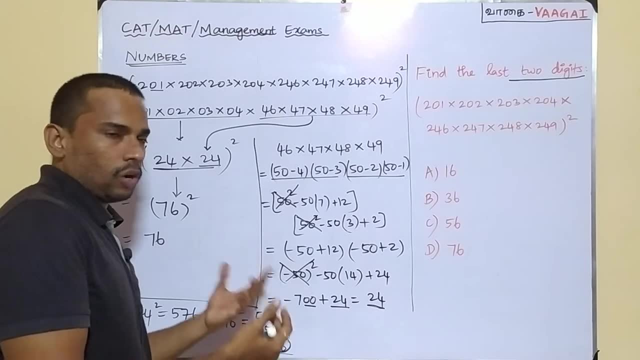 is going to end up with the two digits, which is again 76. that's it okay. so that means these many steps we need to undergo- i mean perform- in order to get the answer? okay, so we are going to do this, and, of course, this is not the only way to solve the problem. of course, there are many other. 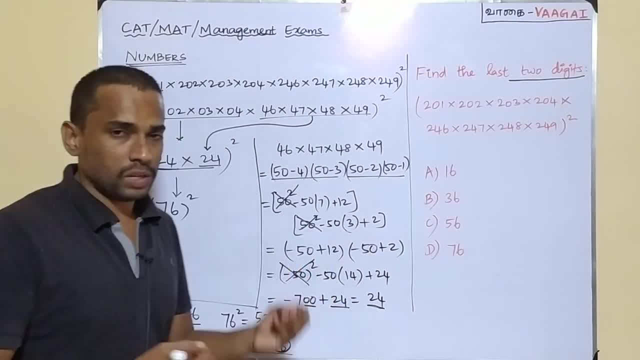 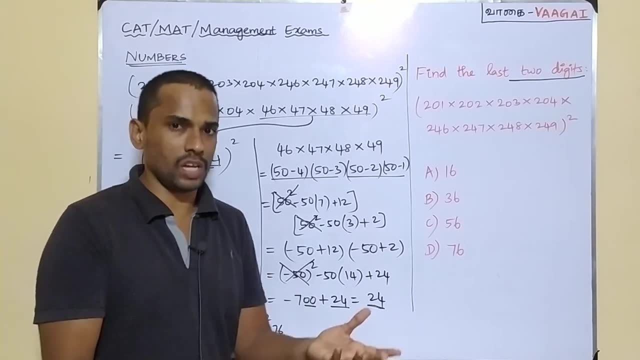 approaches. there are little bit advanced approaches. also, if you are much clear with algebra's basic concepts- and more and more formulas of course- i assure you can finish off this problem in a more easier way. i will. i will tell that. so it is not that this is the 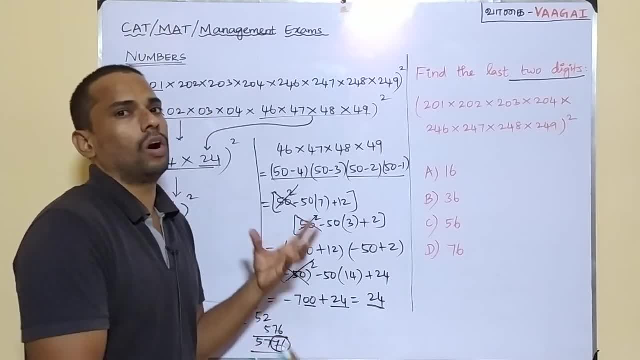 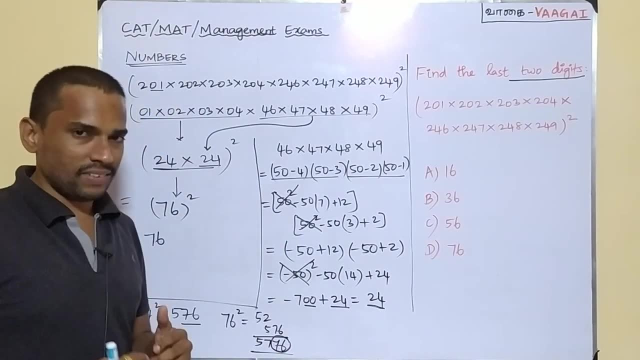 only way to solve the problem. this is just one such approach in order to solve this problem, to get the answer, and of course, that is what we are carrying out- and getting the answer. so your final answer is going to be: 76 is going to be the answer and, yeah, our answer- 76 is available at option d. option d: 76 is going. 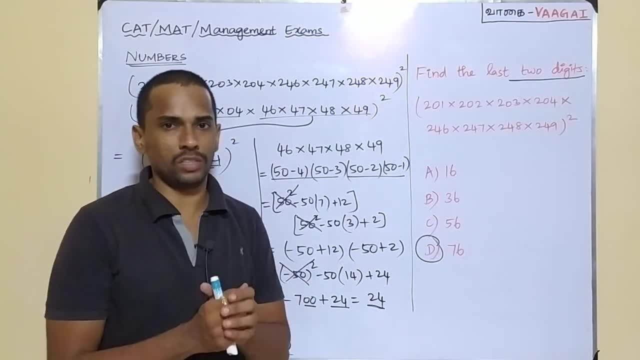 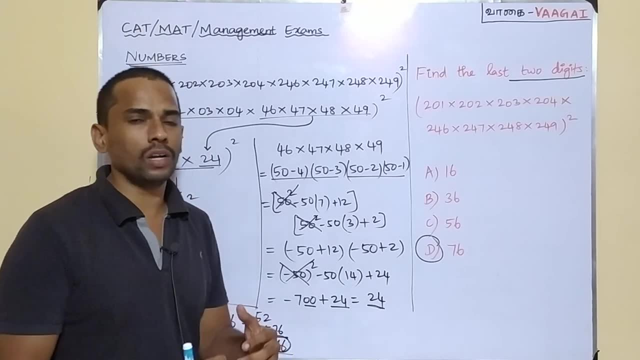 to be the answer for this interesting question. i hope you enjoyed this question and also i hope you are able to understand the procedure, what we carried out here and if at all you get any doubts here, you are most welcome to comment in the comment box and when i see it i'll see to. 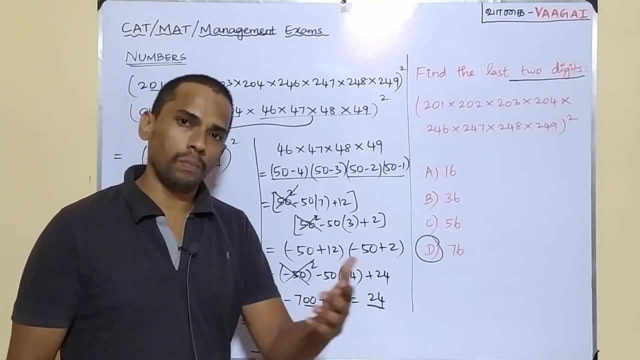 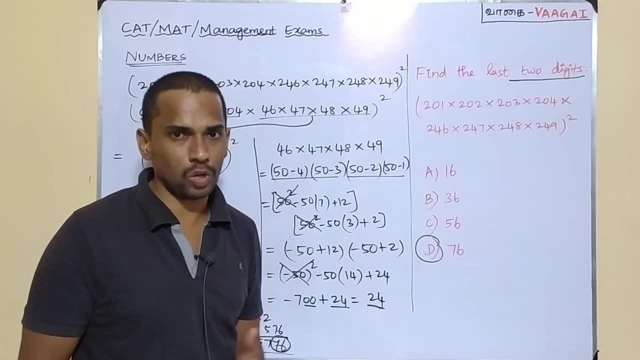 rectify your doubts. okay, and if you feel this session to be useful, please give a like and, as usual, if you feel this would help any of your friends, please do forward. please do share the video to your friends also. again, we'll catch up in the next video with some other interesting questions. see you soon there. thank you so much.